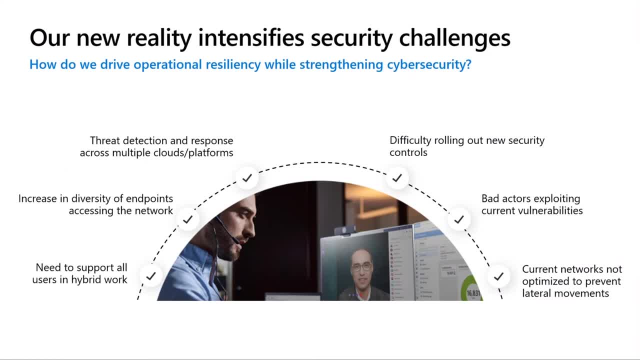 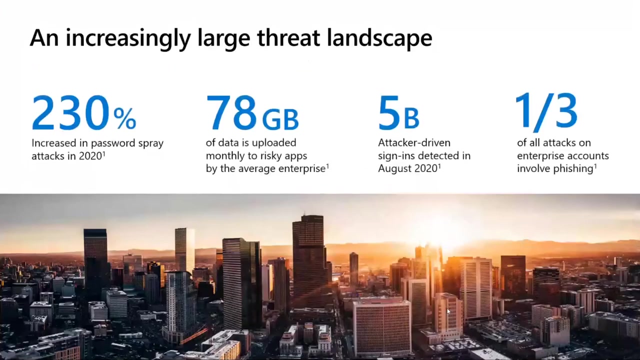 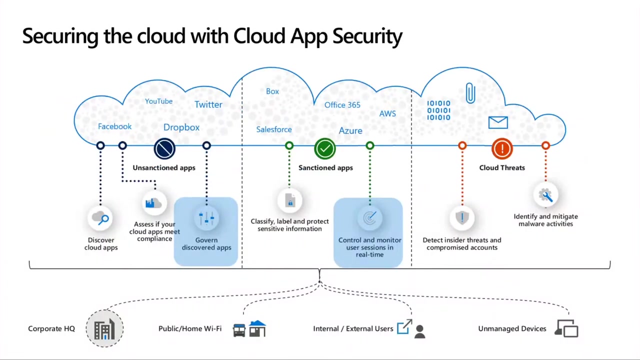 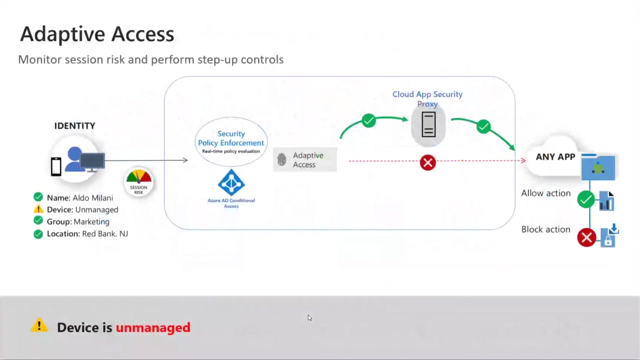 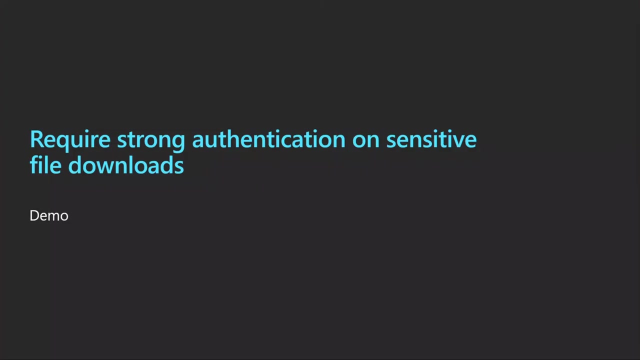 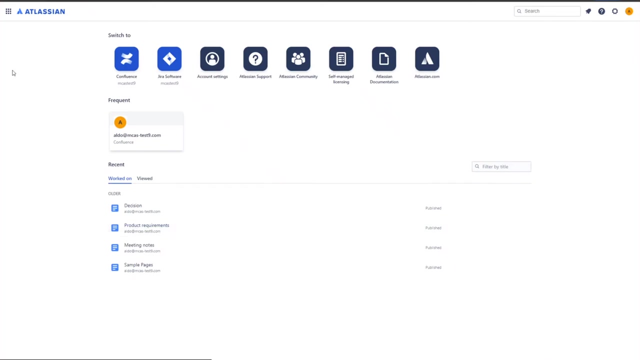 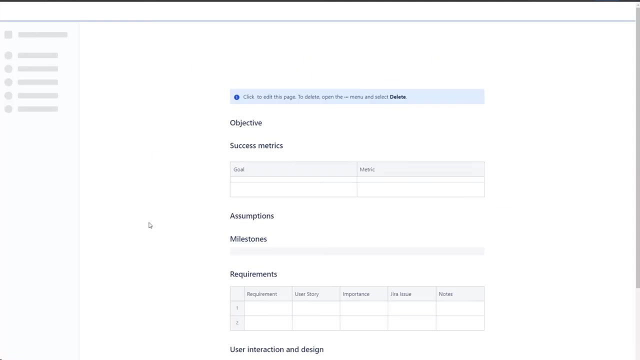 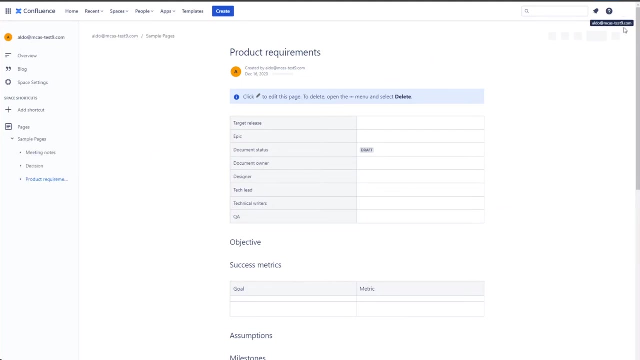 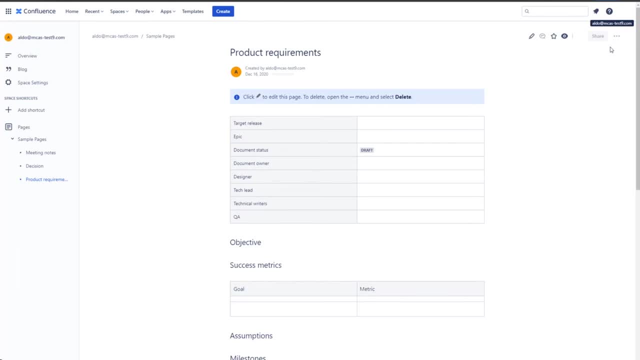 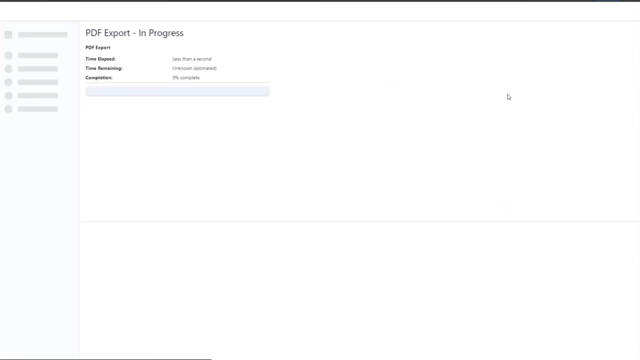 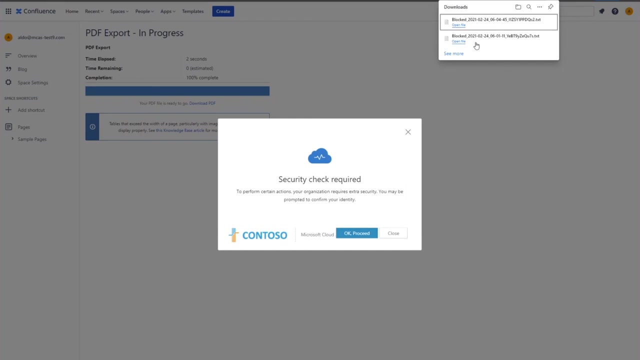 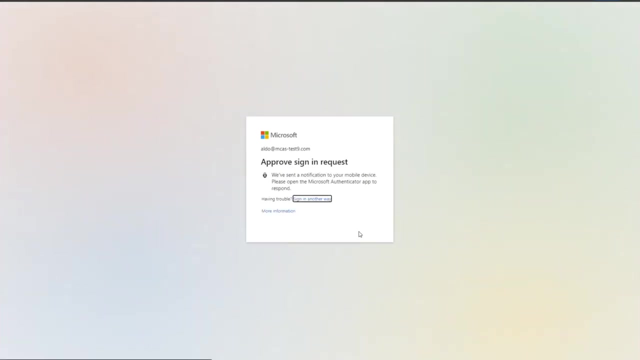 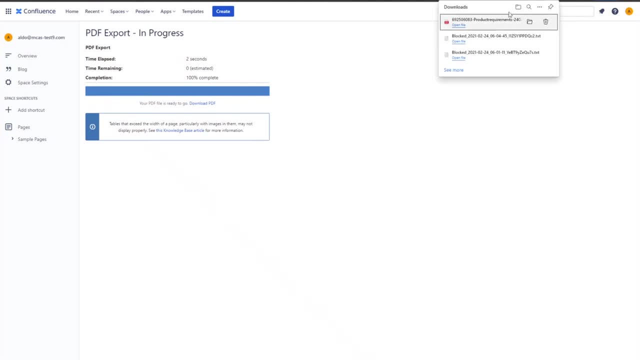 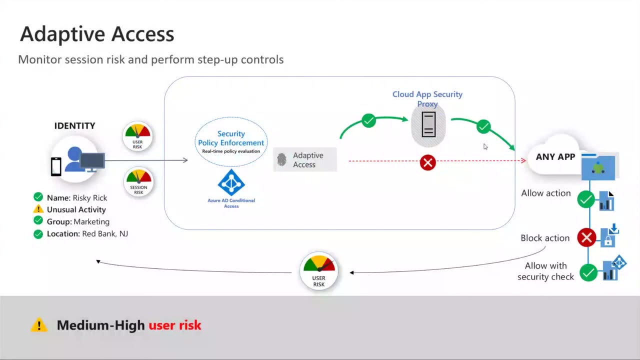 When I download that PDF, in the top right-hand corner you will see that PDF generate and I'm able to access the file. Well, that was the case for Aldo, because he was coming in from a managed device. What do we have? a user that is experiencing some risky behavior. 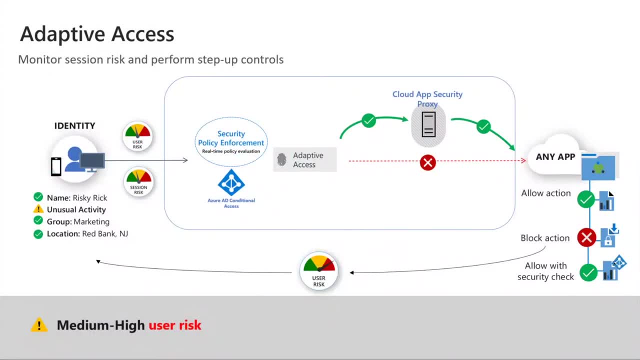 Here we have risky Rick. He's been performing some unusual activity before. What we've seen is that currently his user risk is at a medium and his session risk is also at a medium. He will go through the Azure AD conditional access policy and go through the proxy as expected. 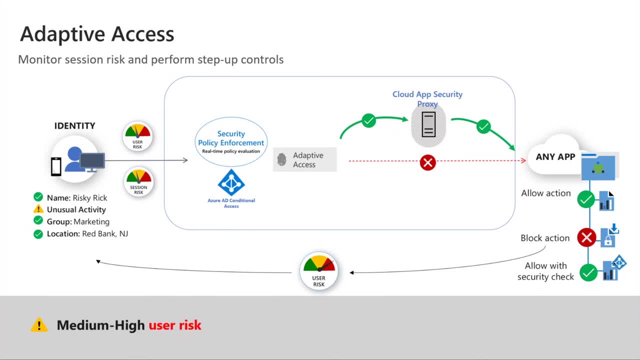 But now any action that he performs will be blocked. as expected. This block action will be signaled directly to the admin, but the admin can then determine whether they want to escalate risky Rick's user score to a high In the next demo. what I will show you are three main components. 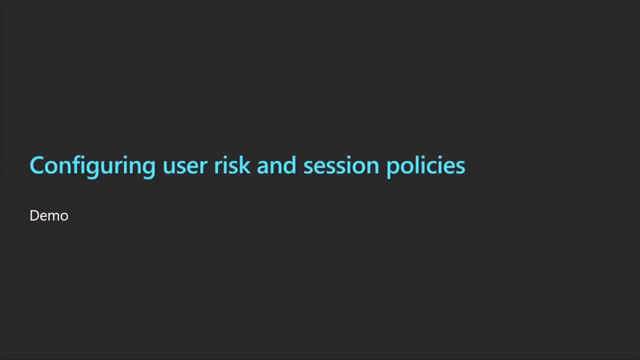 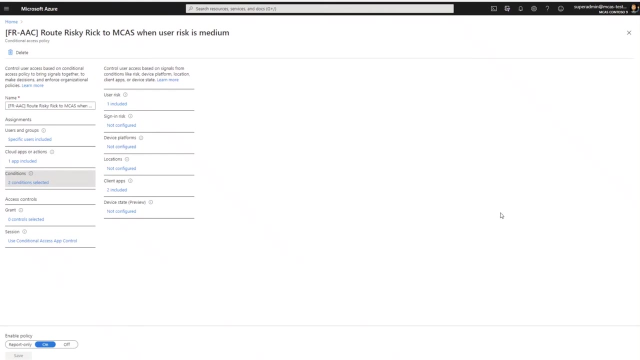 We'll start with configuring the user risk and session policies Here at the user admin. I'm logged into the Azure portal under the conditional access policy, where I'm routing risky Rick to Cloud App Security. when the user risk is medium, I've already selected Rick and 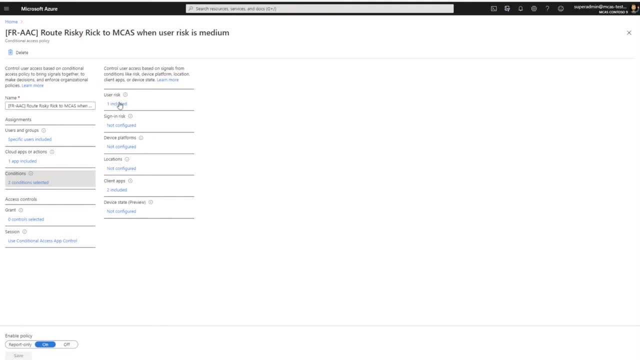 the Cloud applications. I'd like this to apply to and the conditions involved. Specifically, in the conditions, we have user risk and it is at a medium. This user risk is calculated offline based on Microsoft threat intelligence signals, and so this is automatically configured behind the scenes. 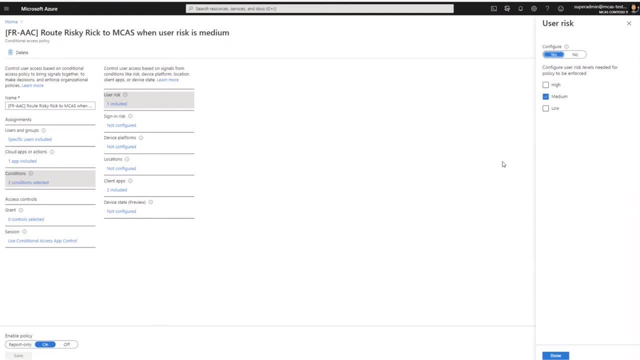 I don't need to do any manual configurations here, unless I, as an admin, would like to escalate his user risk. Then we have the component which allows us to pivot to the Cloud App Security proxy. Here is that single-click integration of use conditional access app control. 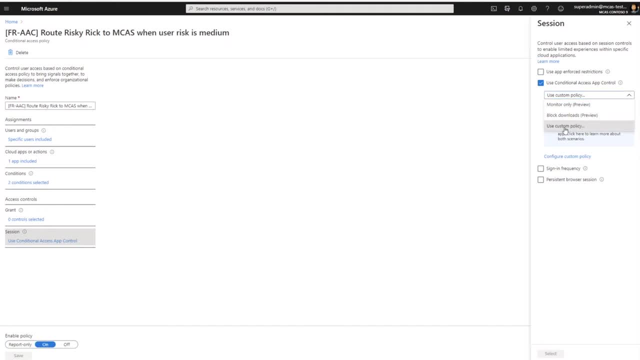 While we can monitor only or block downloads, in this particular case we're going to use a custom policy. What we'll see here is that this policy can be configured directly in the Cloud App Security portal. I've pivoted to the session policy. 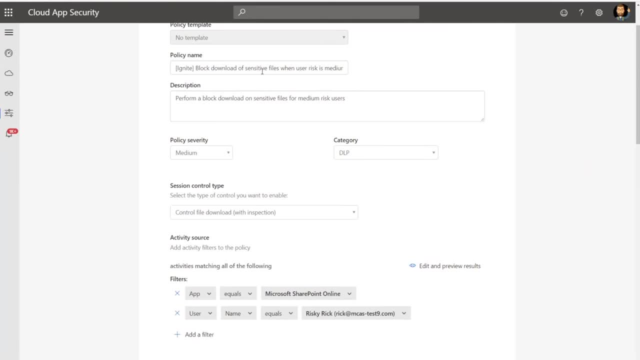 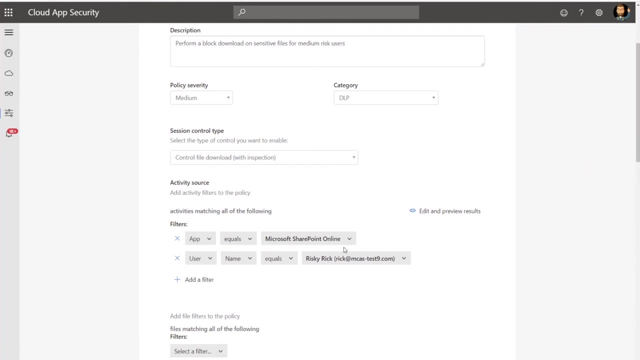 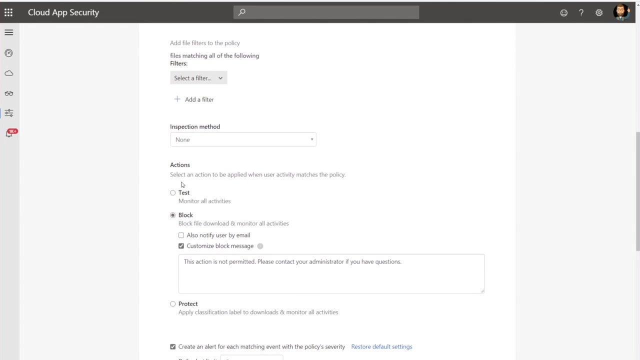 that's configured in the Cloud App Security portal, where I'm blocking download of sensitive file when the user is in medium. specifically for the case of risky Rick, I can select an application filter, username and a plethora of different filters here. As I scroll down, I can select different actions. 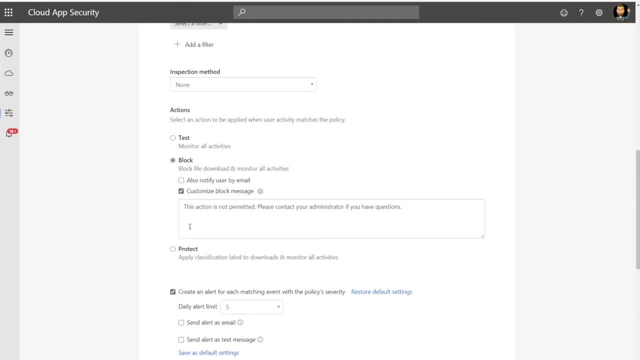 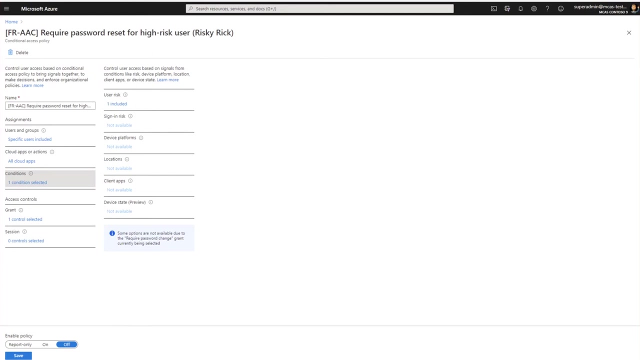 such as test, block or protect. In this case, I am going to block and provide a customized message saying the action is not permitted and to have Rick contact his administrator if he has any questions. The third policy that I'll create is in the case where 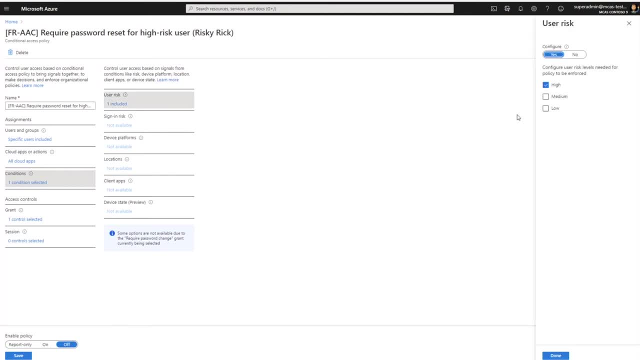 risky. Rick's user risk ends up escalating to high. In this case, this is indicated that Rick has might or might indicate a compromised user. What we'll find here is that a grant control has been applied to require a password change if Rick's account has been compromised. 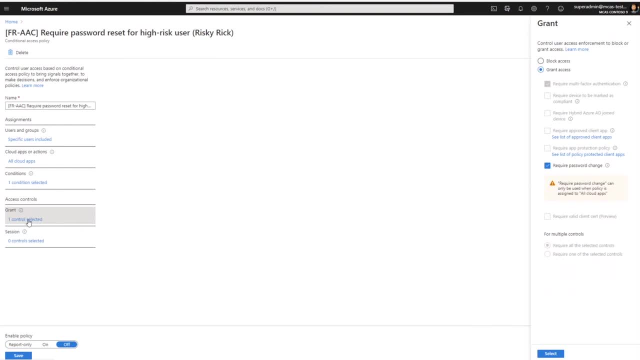 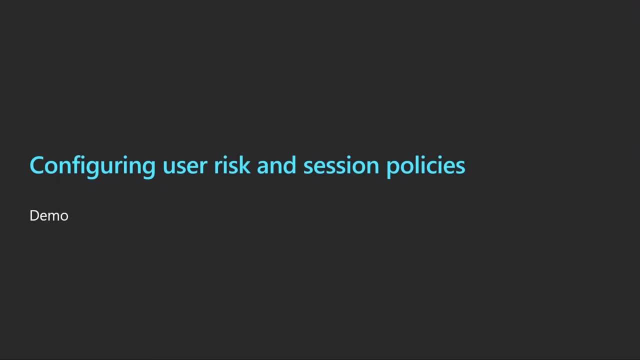 and I as an admin, have escalated that accordingly. Now that we've configured all of the relevant policies, as the admin we'll now pivot to the end user experience. Now we'll see that risky Rick as a current risk of medium and all of the downloads that he. 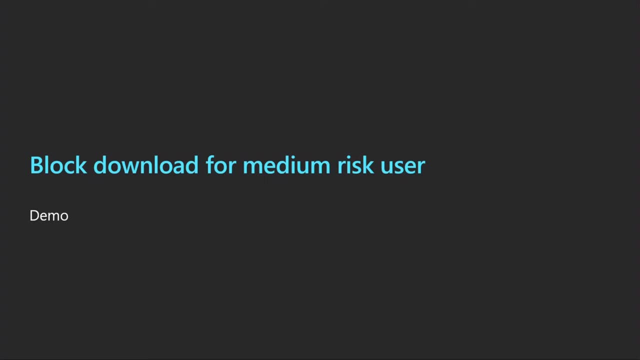 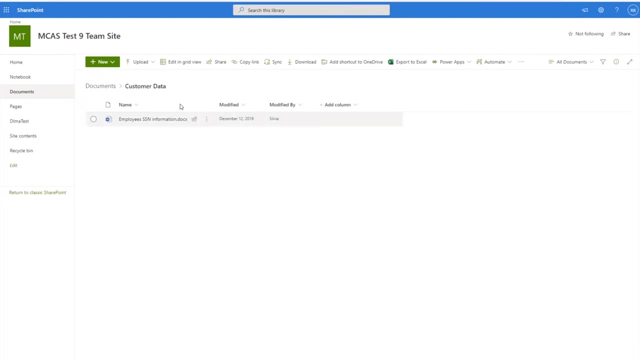 conducts in his environment will be blocked, as expected. Here I'm a risky Rick. I'm logged into our SharePoint site and I viewed a folder of customer data. I'm currently undergoing the Microsoft Cloud App Security reverse proxy, As you can see that. 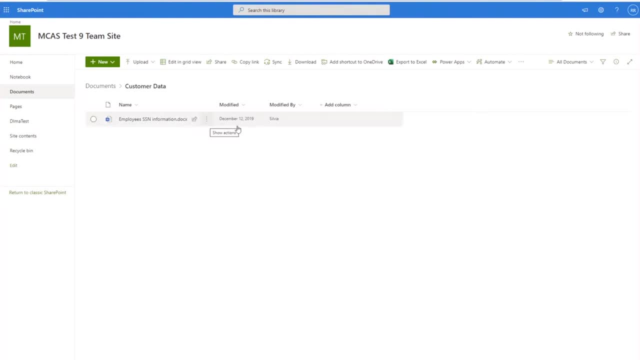 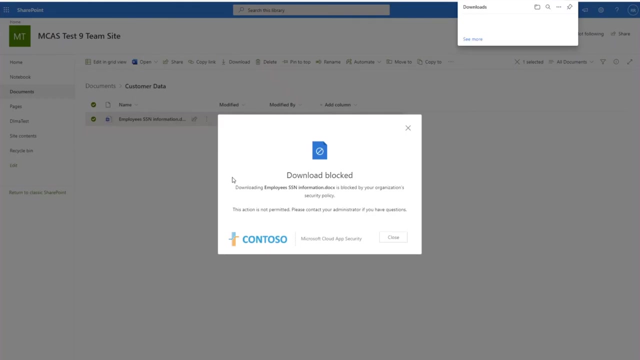 domain is appended Here. I see that Sylvia has uploaded some nice sensitive information of social security numbers. I decided I'm currently performing as a bad actor and I would like to download that specific information. You can see that a tombstone file appears at the top right corner. 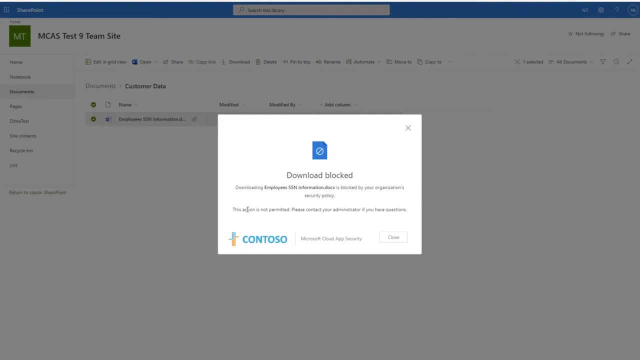 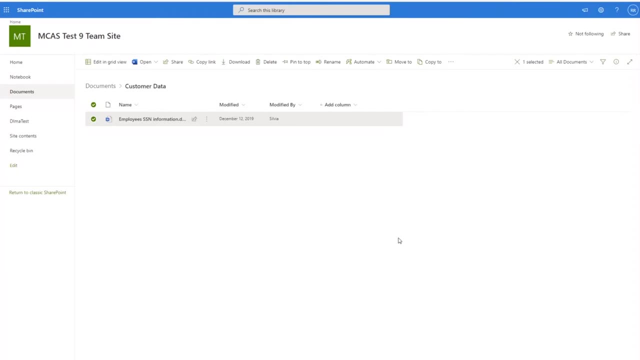 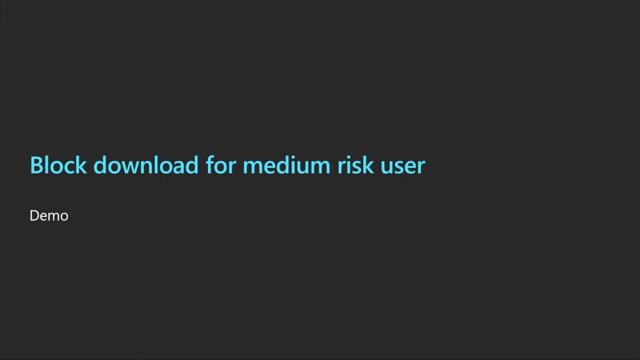 and the download is blocked as expected. There's even a custom message that I showed it before- of this action is not permitted. please contact your administrator if you have questions. So, now that Rick has been blocked from downloading any sensitive content, and if it is, 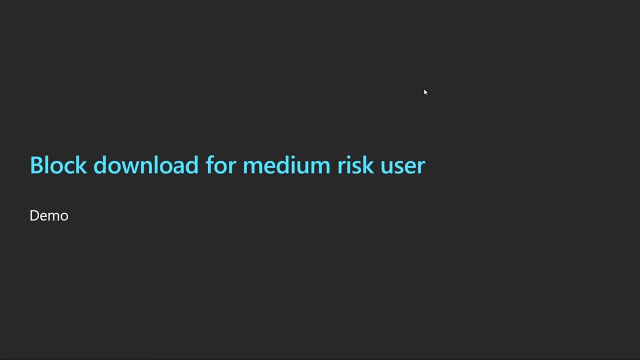 an indicator that he is a bad actor. what we can see is what happens from the admin perspective and we can elevate his user risk from medium to high to require that password reset. We'll pivot back to the admin experience, where there are two things that have happened. 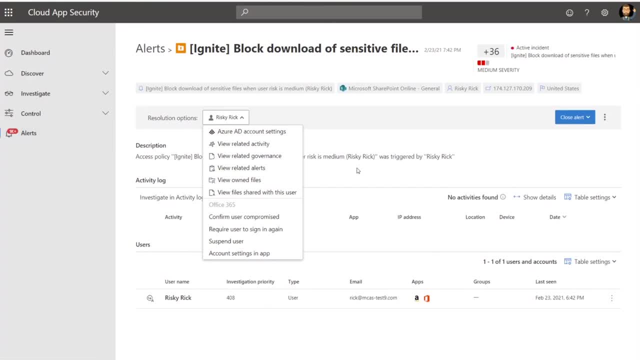 The first and foremost and foremost is that I receive an alert similar to this one where I see a block download of sensitive file where the user is his medium. This is the session policy that I indicated in the beginning and I can actually perform. 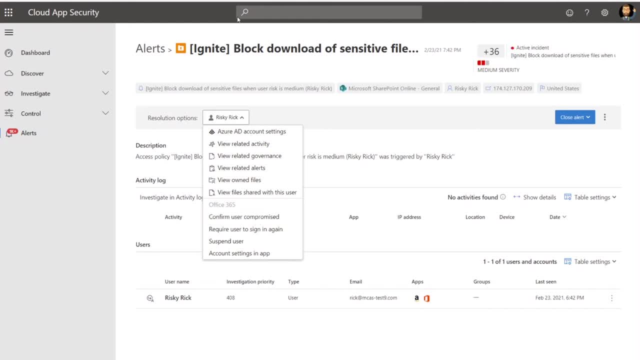 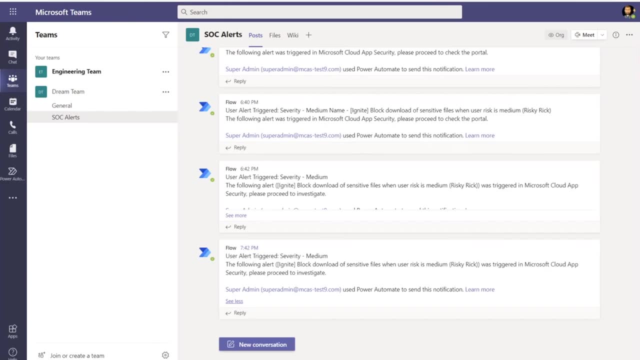 a resolution option right within this alert, right here. But let's say that I don't check my Cloud App Security Console as often as I do with Teams. I can also configure a specific alert that ends up triggering within Teams. that tells me: hey, there's a user alert triggered. 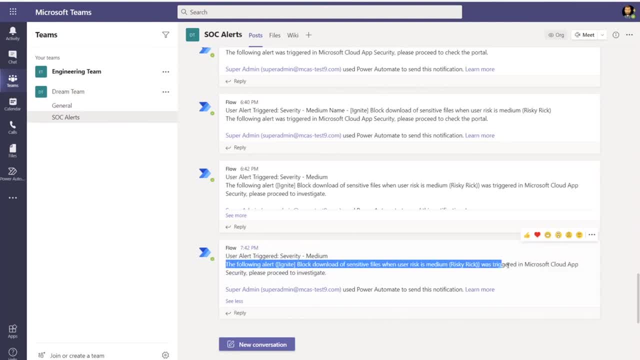 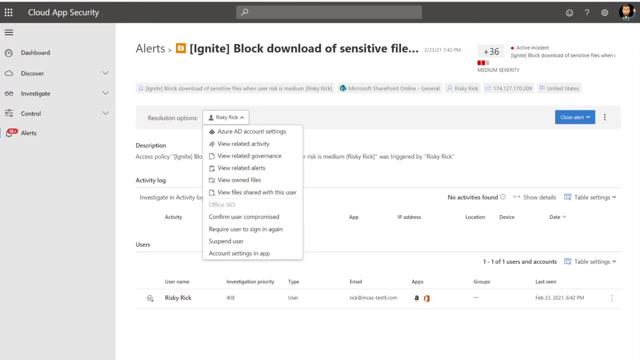 the severity is medium and it gives me more context around the alert. This can be customized as expected as well. Then what happens is that once I actually go and perform that resolution of confirm user compromised, that will immediately escalate risk from a medium to a high. 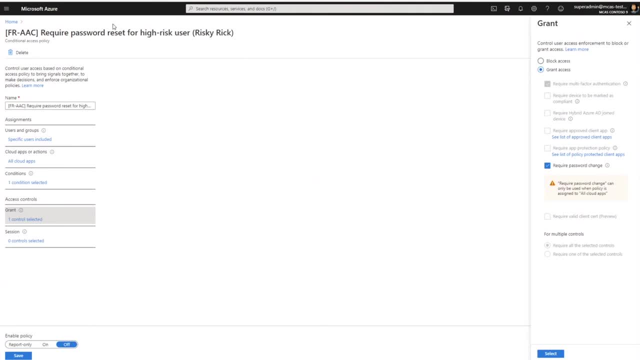 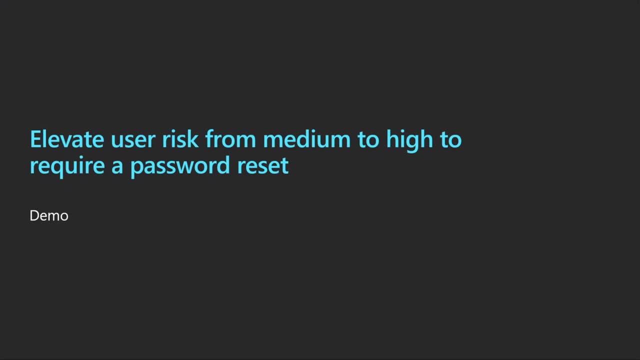 and then it will enforce that policy that I have to require that password reset. I want to take a moment to pause here and just talk a minute about the powerful capabilities that were just demoed, Starting with not only understanding risky RIC and the unusual behavior activity. 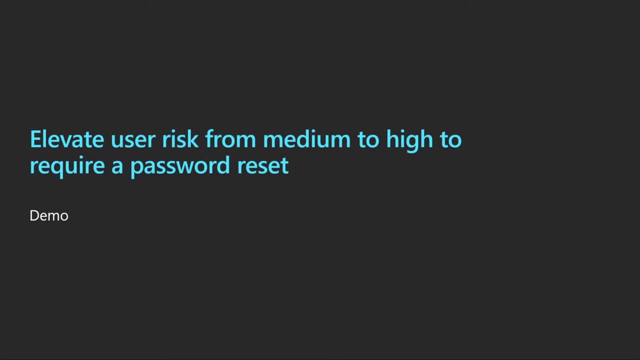 that we initially saw from Microsoft Cloud App Security. we're also able to see that his user risk score was already elevated to a medium status via Azure AD and those Microsoft threat intelligence signals. From there, we were able to take it one step further and create 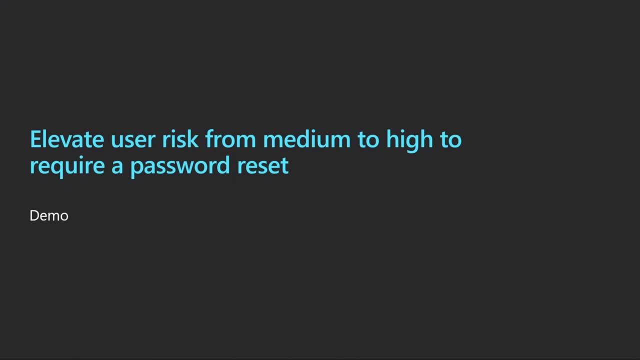 a conditional access policy and a corresponding MCAS session policy to enable this comprehensive session controls to block a download if any sensitive actions were performed, Then we took it one step further from the super admin perspective to understand. not only was that sensitive action blocked, 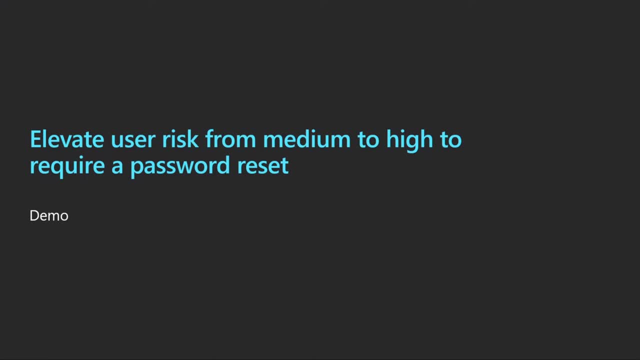 but it was alerted upon and alerted upon to the extent of Teams and directly into the SOC channel. As a super admin I was able to go in and directly escalate risky RIC's user risk from medium to high to require that password reset. 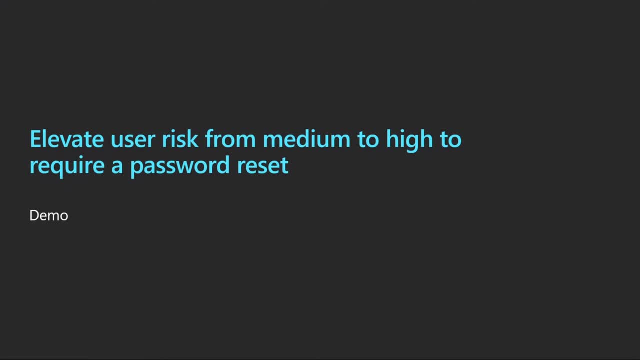 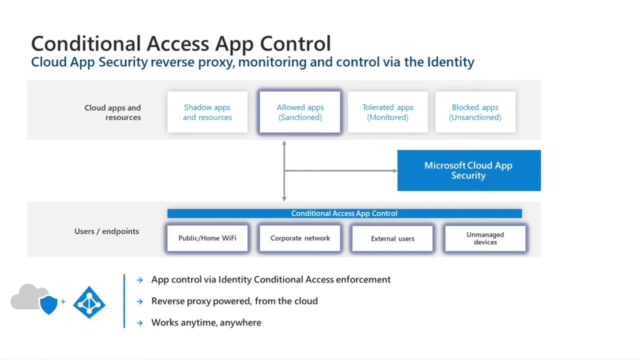 that policy that I enabled right from the get-go. So this really, really showcases the power of conditional access, app control, the power behind the reverse proxy, the ability to add access and session controls. One thing to note for both the ALDO and risky RIC scenarios. 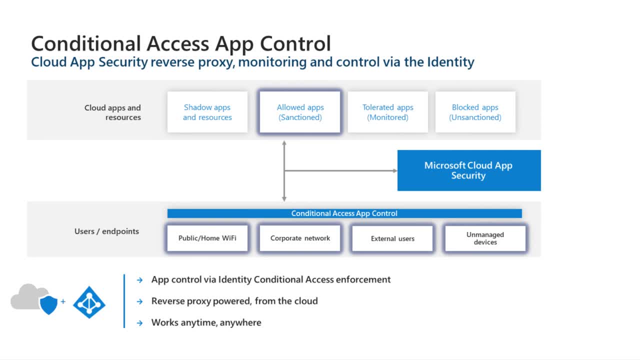 is that these were configured for sanctioned applications. They were both single sign-on configured applications that were available in the Azure AD app gallery and we extended off of that conditional access integration to apply those session controls, apply that block download and step up accordingly. 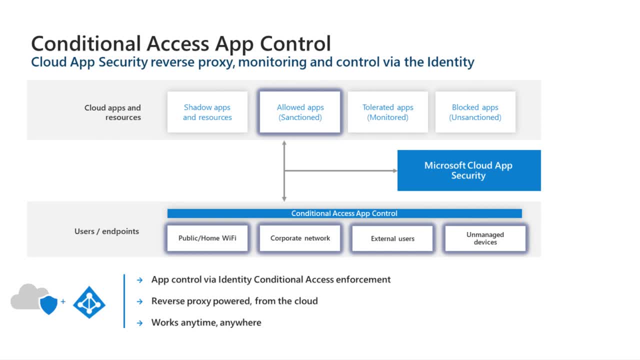 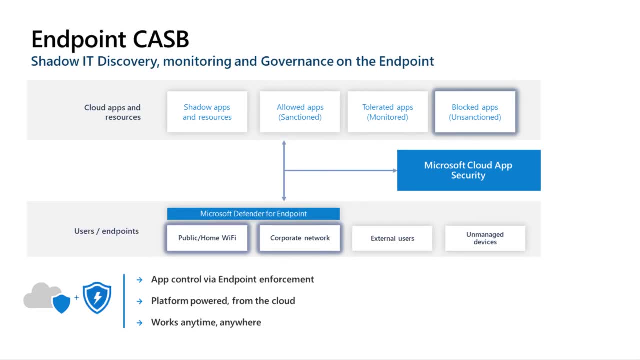 While this does work anytime and anywhere, we are still missing the scenarios around unsanctioned apps. So what do we do? Well, we can leverage another technology within Microsoft Cloud App Security, which is the Endpoint, CASB. This leverages the shadow IT discovery feature. 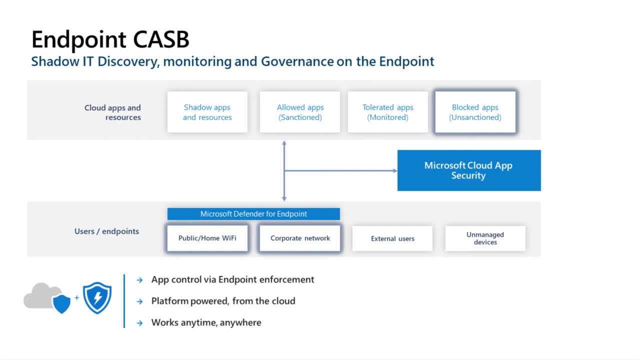 which allows us to monitor all of the different Cloud applications that exist in our ecosystem and also apply governance actions via Microsoft Defender for Endpoint, Again, this is a simple single-click integration where we're immediately able to get recognition of the applications users IP addresses. 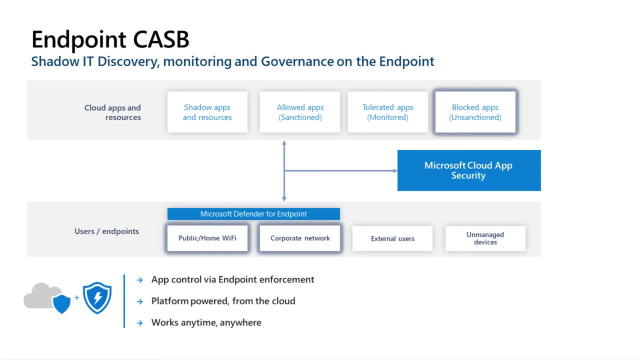 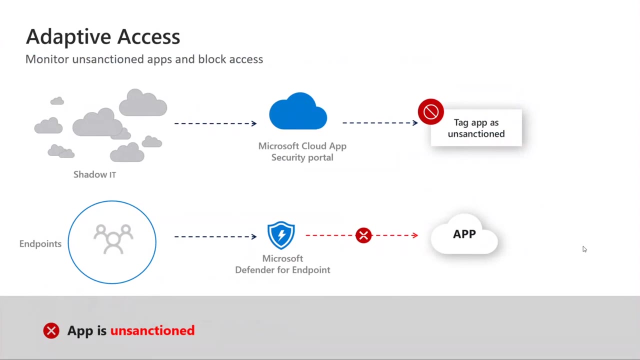 and even devices that are accessing these endpoints from the home, Wi-Fi or corporate network. It works anytime and anywhere as well, and it's all powered from the platform, from the Cloud. How does adaptive access tie into Endpoint CASB? At the top we have that shadow IT. 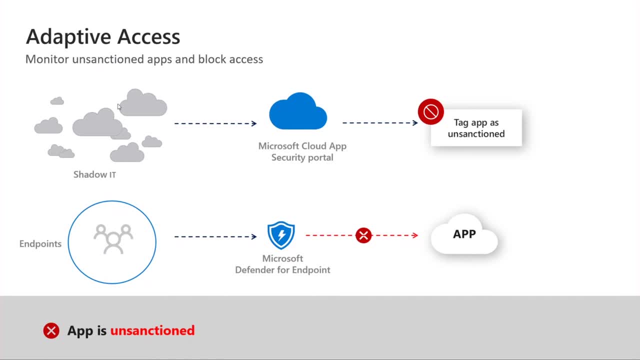 These are all of the applications that we might be unaware of as an admin of what our employees are accessing day-to-day. Luckily, that shadow IT is aggregated and parsed in the Microsoft Cloud App Security portal, So we're able to see all of the different applications displayed. 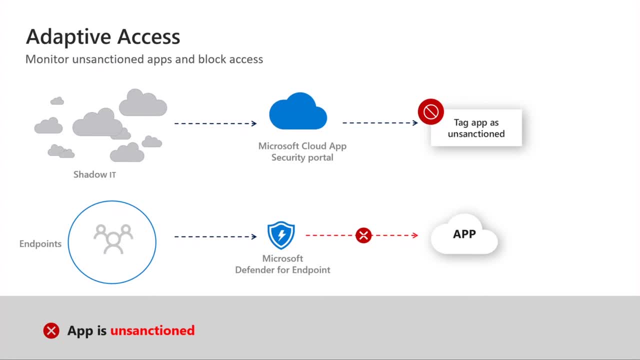 and then tag those applications as sanctioned or unsanctioned. Then from the end-user perspective, wherever that end-user is coming from the endpoint for that corporate managed device, typically they'll have that agent installed for Microsoft or Microsoft Defender for Endpoint. 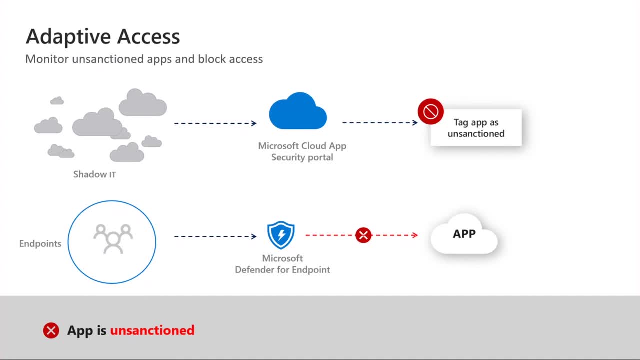 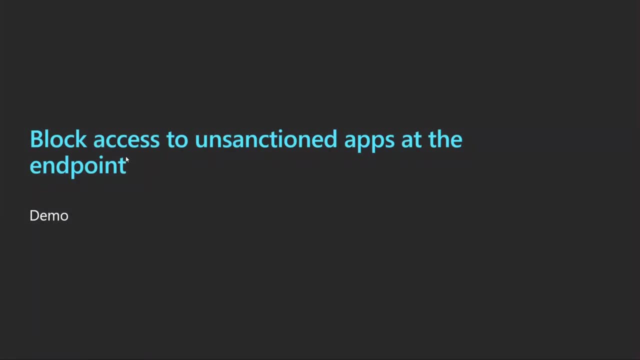 Any application that's tagged as unsanctioned would be blocked, and so they're not able to access that specific app. Instead of me going through that scenario, let's actually see that in action. I'll break this down into the top layer and bottom layer, as I described. 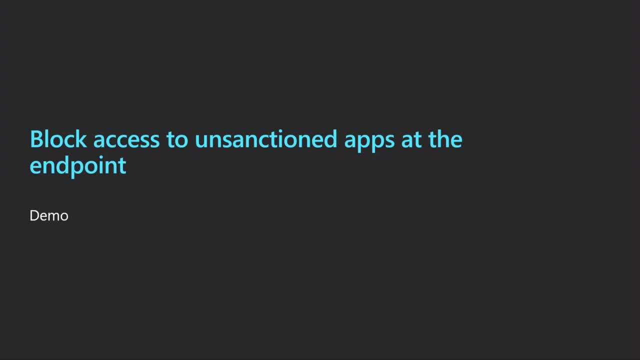 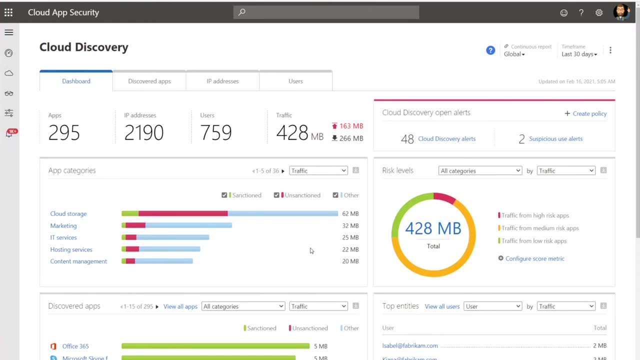 First and foremost, with that admin experience As Safer Admin, I'm going through our Cloud Discovery Dashboard and I immediately have visibility in the apps: IP addresses, users, traffic, all of that information. This is our global report, If I pivot to our Microsoft Defender for Endpoint report. 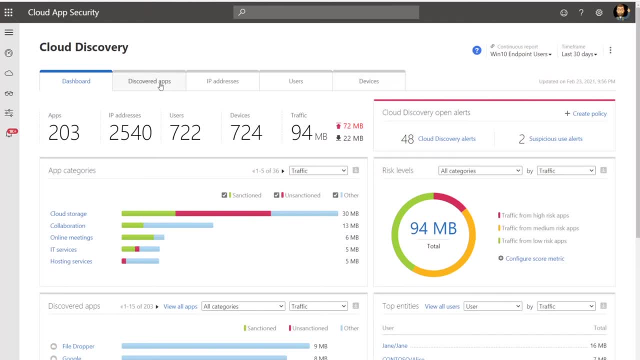 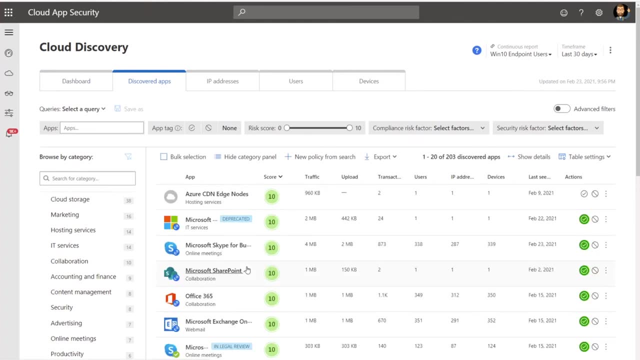 I also get an additional tab of devices right here Now. if I go into our discovered apps, we'll see all of the different applications that were recognized just from the endpoint alone. So all of these applications are sanctioned. they seem to be a very low risk. 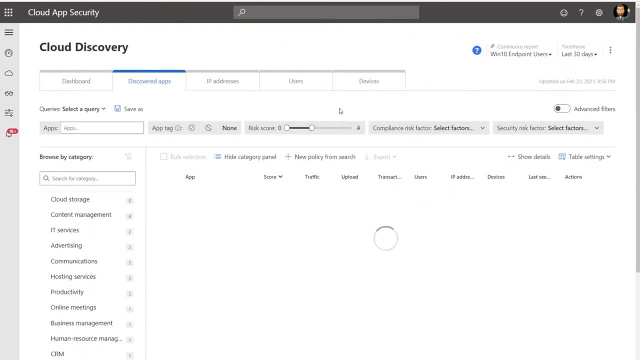 Let's go to some of the high-risk applications First and foremost. what we'll see is Backblaze, which is a Cloud Storage application, has a risk score of four. If we extend this to understand, why was it scored as such? 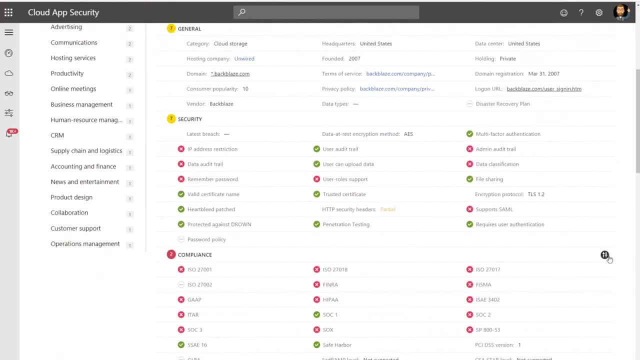 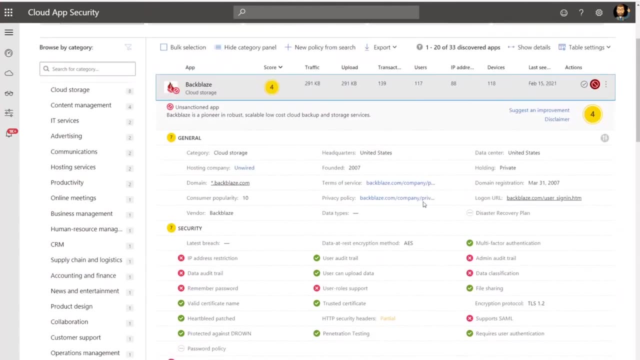 we'll have a general security and a compliance rating. We can even adjust these score metrics to understand and say: this is what matters for my company and how I would like this risk score to be leveraged For the purpose of this, being a third-party Cloud Storage. 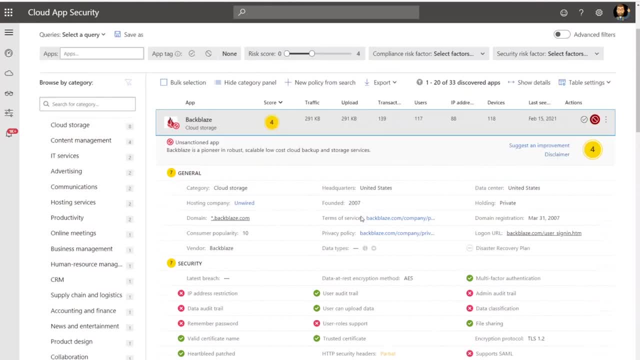 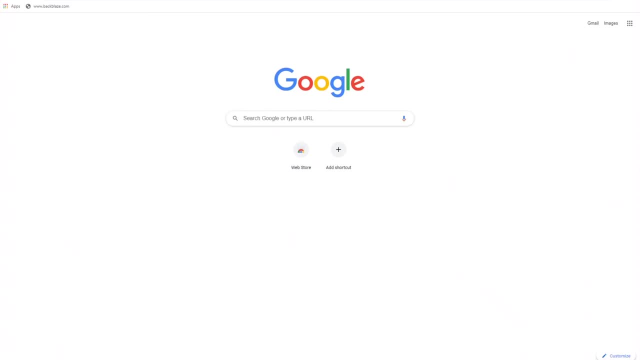 we have already unsanctioned this application, So any end-user that was accessing this will not be able to do so. So let's see that in action. So I quickly pivoted and now I am an end-user, Jane, My device information and everything is in the portal. 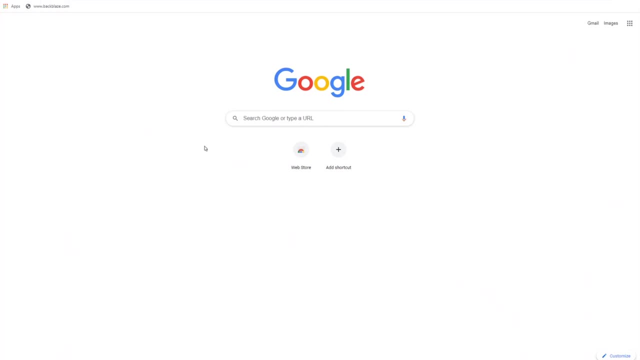 What I want to do is access that Backblaze application. What you'll see in Chrome is that access to Backblaze was denied and we get a warning. Okay, So now we're going to get another Windows Security notification that says the content was blocked. 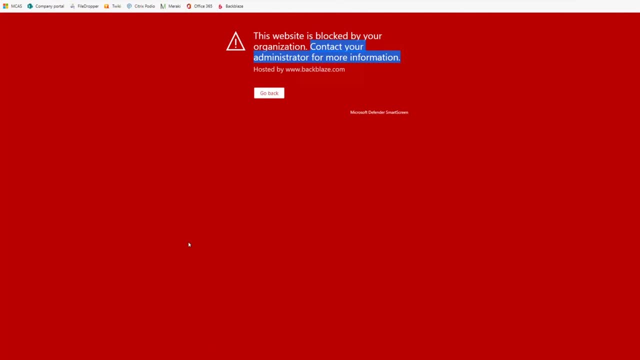 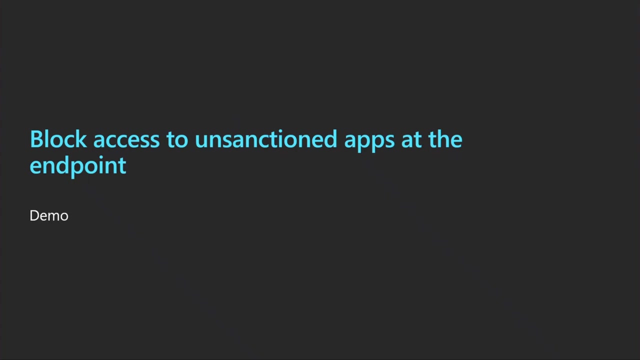 In Microsoft Edge Chromium, we'll see something very similar, where we have a Microsoft Defender Smart Screen taking place where the website is blocked by the organization and that I should contact my administrator for more information. Now that I've showcased both the admin and end-user experience, 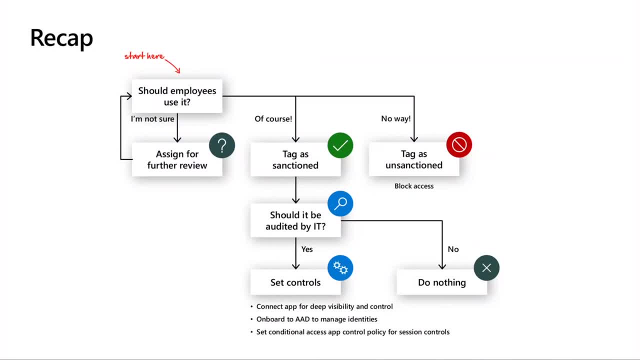 we're going to have a little bit of of the overall adaptive access scenarios we covered, So I showcased two scenarios specifically with sanctioned applications and one with the unsanctioned application. In general, any application that's tagged as unsanctioned should be audited by IT if needed. 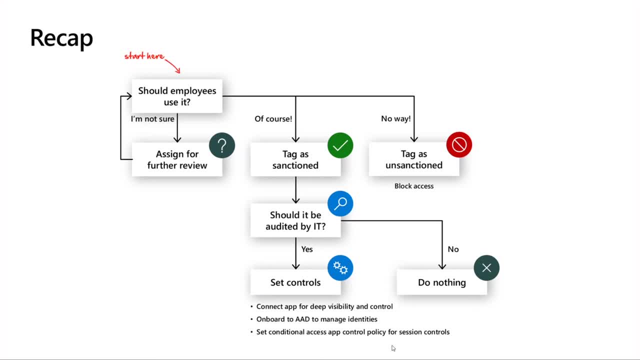 and control should be applied accordingly. We saw that power of Conditional Access App Control, the ability to block a download in real-time, being able to perform a required MFA challenge when a download is done was happening. There's a lot of different nuances and 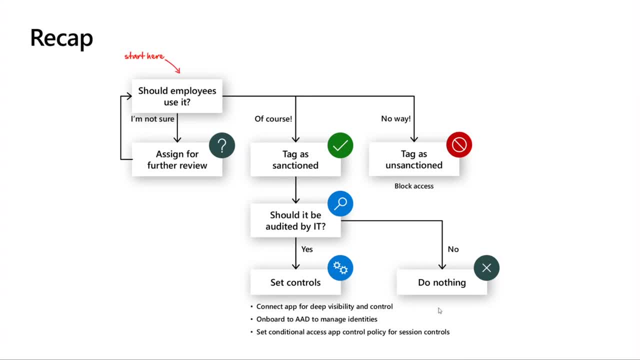 powerful integrations right within the control aspect, But for any application that's not compliant with the company, it's best to just block access immediately. So you can do that from the endpoint or other scenarios, such as generating a block script or even leveraging Secure Web Gateway integrations if needed. 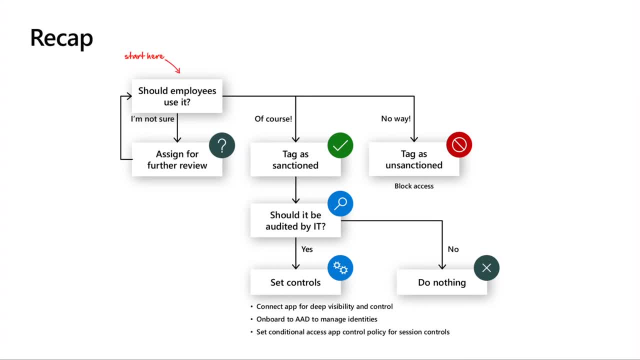 Now this all ties together in the story of now that you are an admin and would like to understand your Cloud landscape. Now you need to consistently ask yourself the question of: okay, I've discovered this application. should my employees use it? 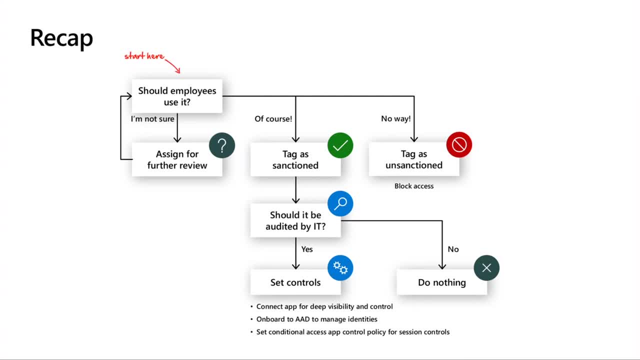 So this table helps guide you to understand. well, yes, then tag the app as sanctioned. no, then tag the app as unsanctioned. We do understand there are more nuances and we're continuing to build on top of this base foundation here.